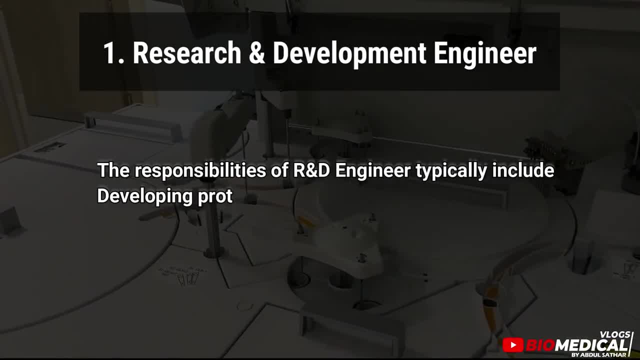 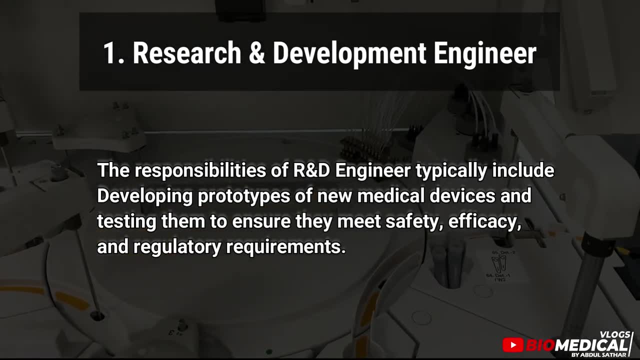 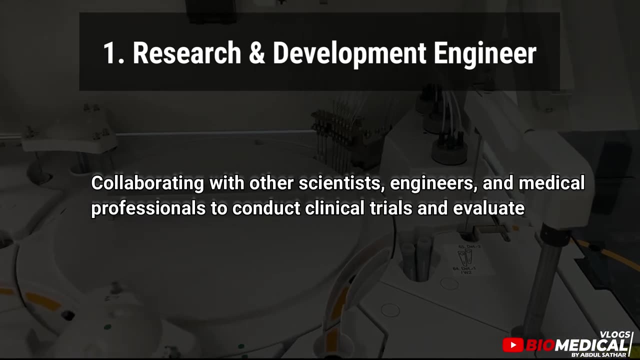 The responsibilities of a R&D engineer typically include developing prototypes of new medical devices and testing them to ensure they meet safety, efficacy and regulatory requirements. Collaborating with other scientists, engineers and medical professionals- local doctors and medical professionals- to conduct clinical trials and evaluate the effectiveness of new medical devices, etc. 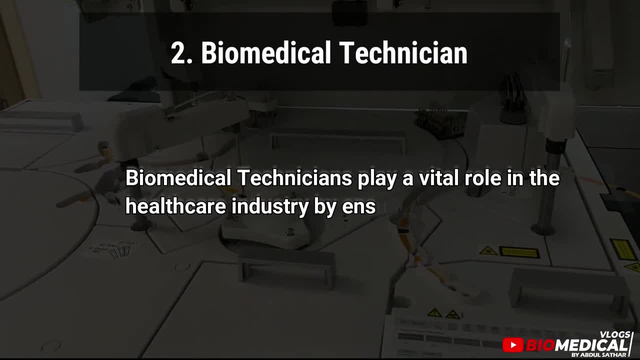 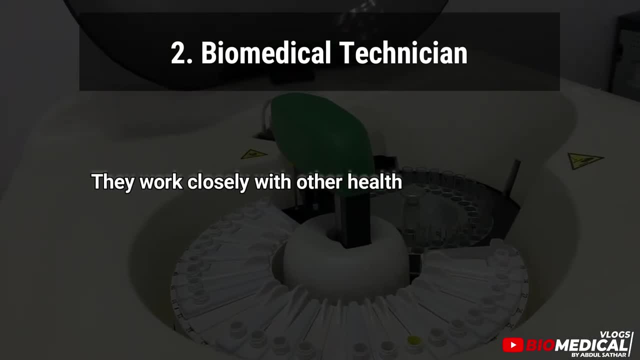 2. Biomedical Technician. Biomedical technicians play a vital role in the healthcare industry by ensuring that medical equipment is functioning correctly and safely. They work closely with other healthcare professionals, including biomedical engineers, physicians and nurses, to ensure that patients receive high-quality care. 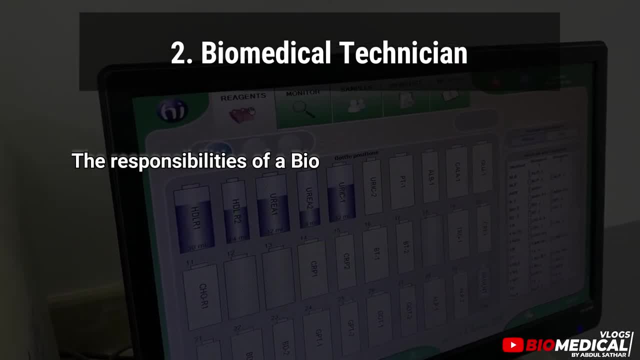 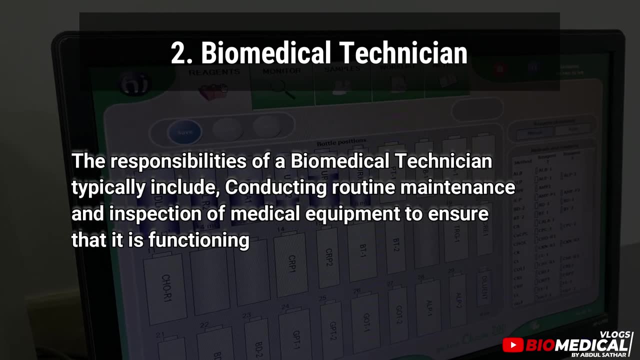 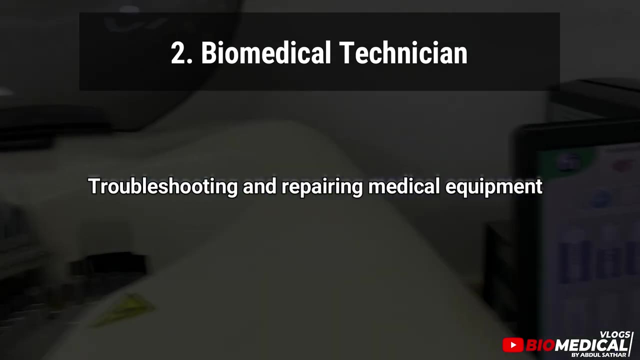 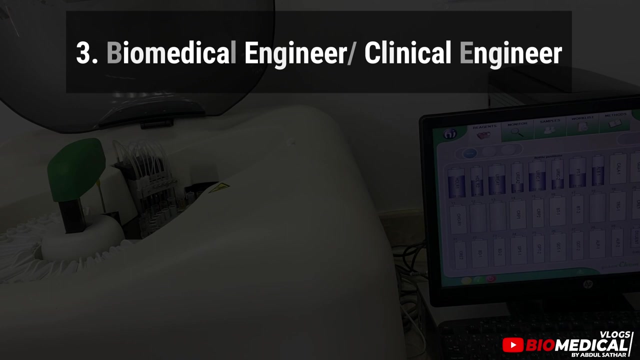 high-quality care. the responsibilities of a biomedical technician typically include conducting routine maintenance and inspection of medical equipment to ensure that it is functioning correctly and meet safety and regulatory standards, troubleshooting and repairing medical equipment and devices that are malfunctioning or not functioning correctly, etc. 3. biomedical engineer or 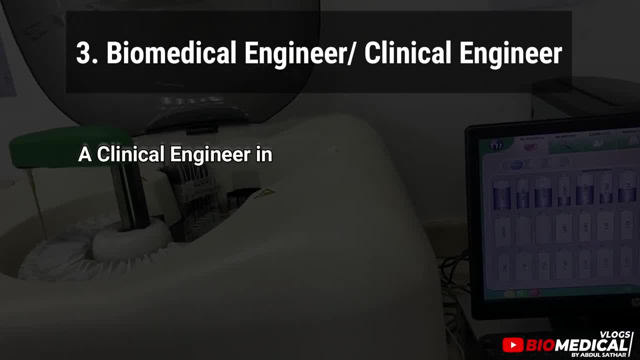 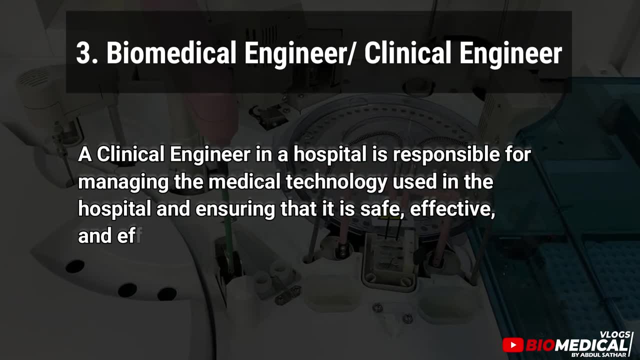 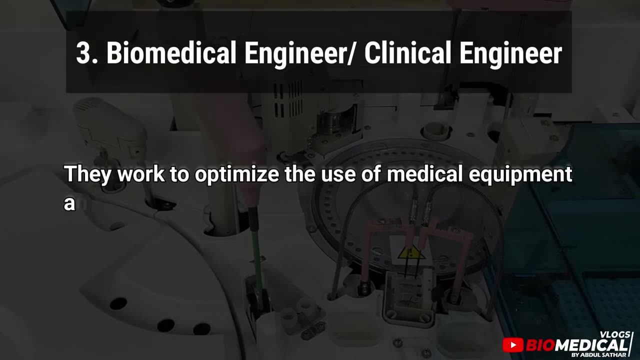 clinical engineer. a clinical engineer in a hospital is responsible for managing the medical technology used in the hospital and ensuring that it is safe, effective and efficient in meeting the needs of patients and health care providers. they work to optimize the use of medical equipment and devices, while ensuring that they are maintained and functioning correctly. the 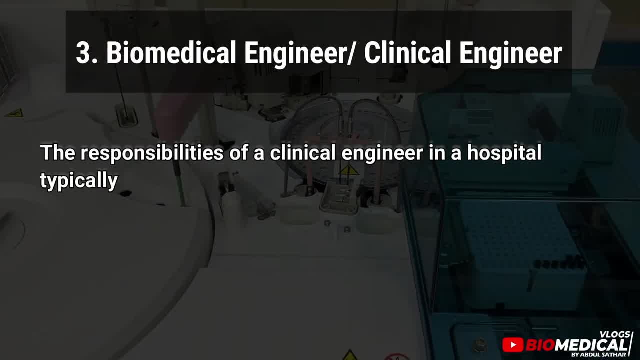 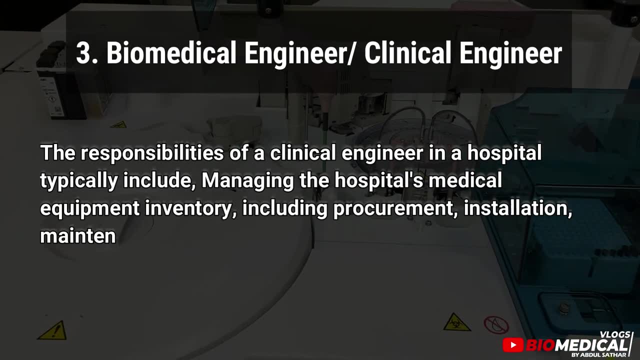 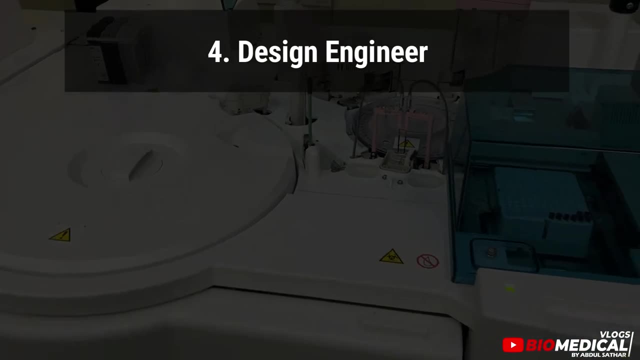 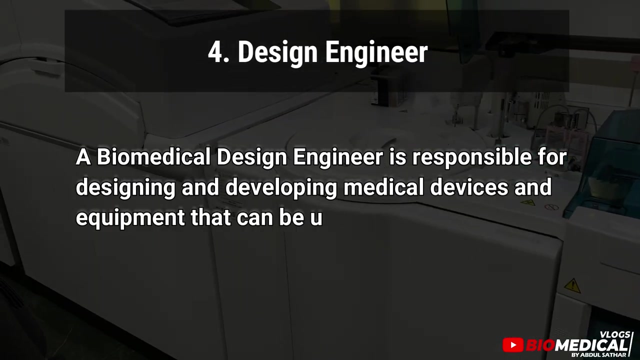 responsibilities of a clinical engineer in a hospital typically include managing the hospital's medical equipment inventory, including procurement, installation, maintenance and decommissioning of medical equipment. for design engineer: a biomedical design engineer is responsible for designing and developing medical devices and equipment that can be used to diagnose, monitor and treat patients. the 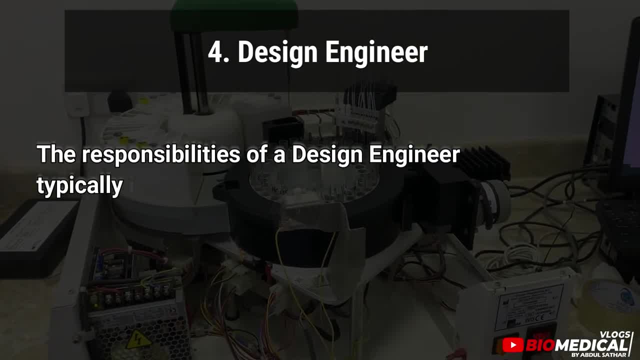 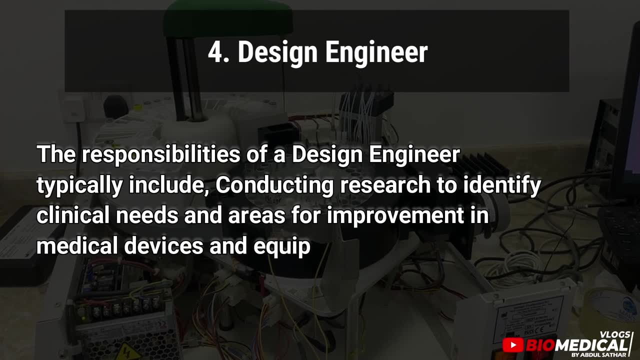 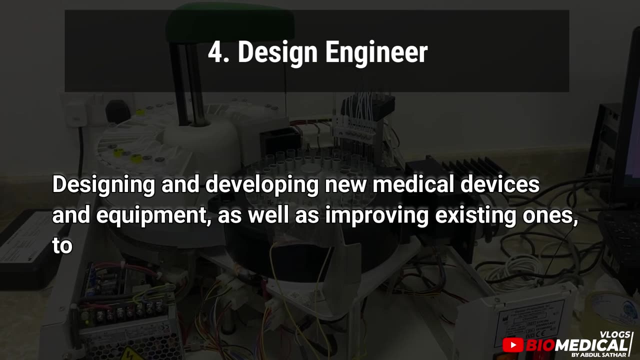 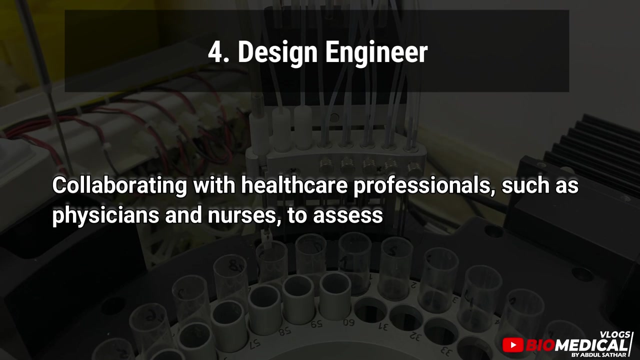 responsibilities of a design engineer typically include: conducting research to identify clinical needs and areas for improvement in medical devices and equipment. designing and developing new medical devices and equipment, as well as improving existing ones to meet clinical needs. collaborating with health care professionals, such as physicians and nurses, to assess the usability and effectiveness of medical devices. 5 field. 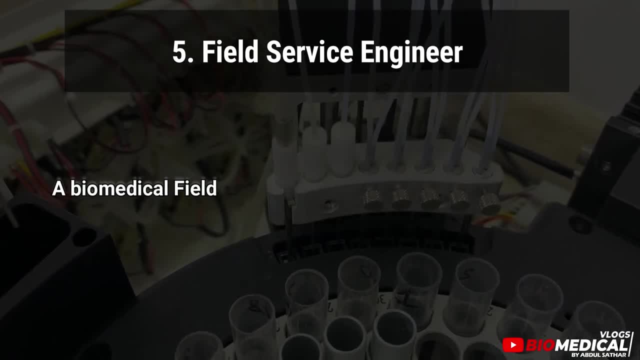 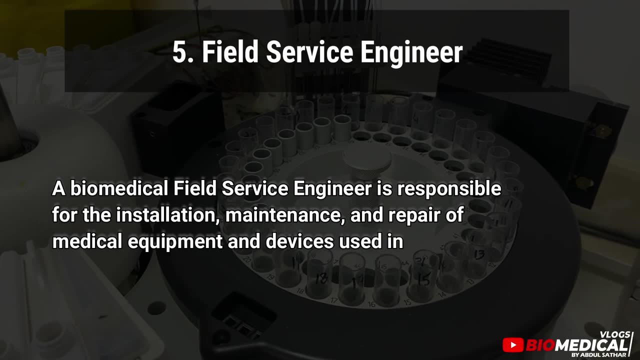 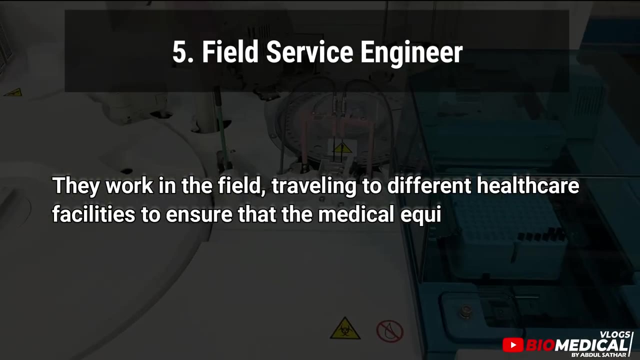 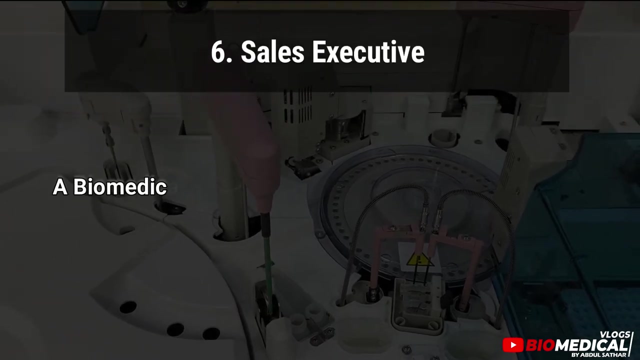 service engineer. a biomedical field service engineer is responsible for the installation, maintenance and repair of medical equipment and devices used in health care facilities. they work in the field, traveling to different health care facilities to ensure that the medical equipment is functioning correctly and safely. six sales executive: a biomedical sales executive is responsible for 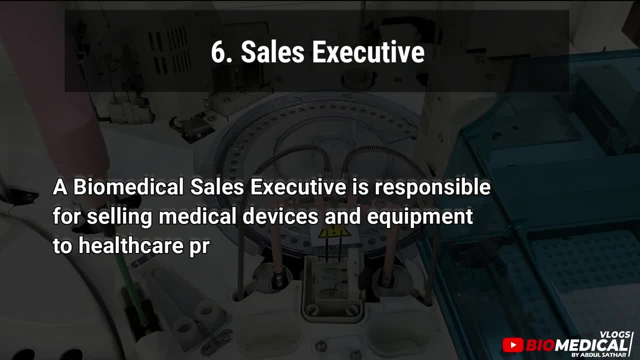 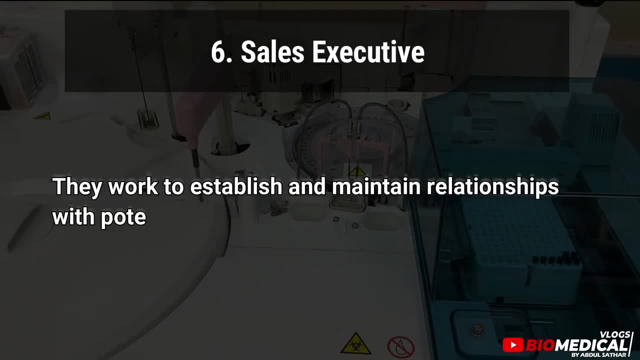 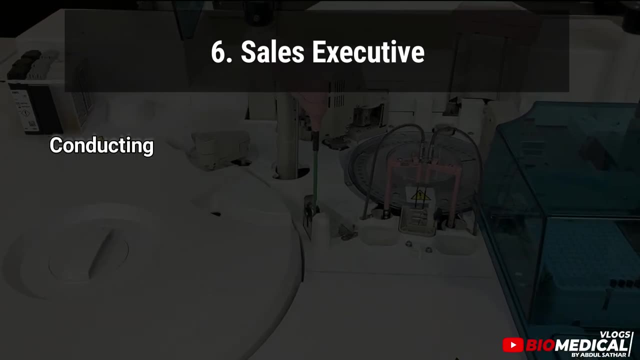 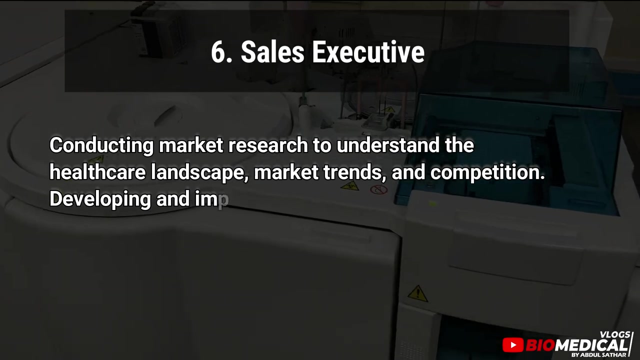 selling medical devices and equipment to health care providers such as hospitals, clinics, etc. they work to establish and maintain relationships with potential and existing clients, understand their needs and provide solutions that meet those needs, conducting market research to understand the health care landscape, market trends and competition. developing and implementing sales strategies to 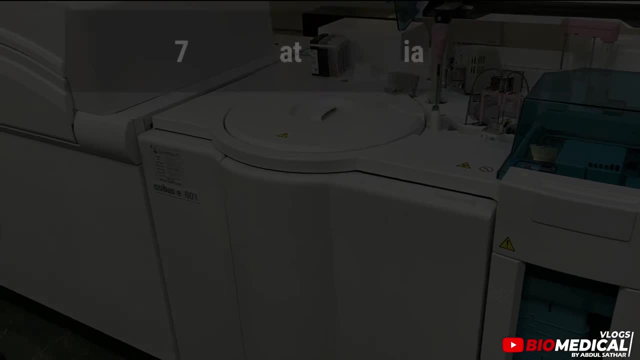 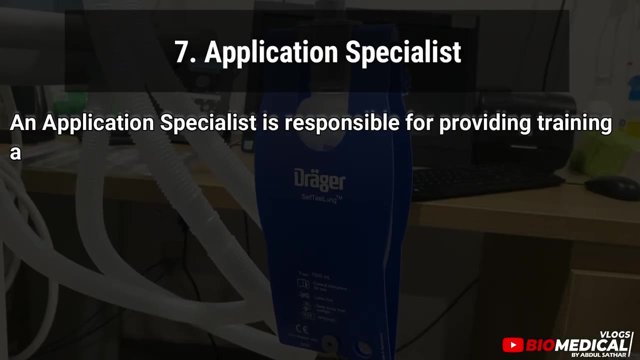 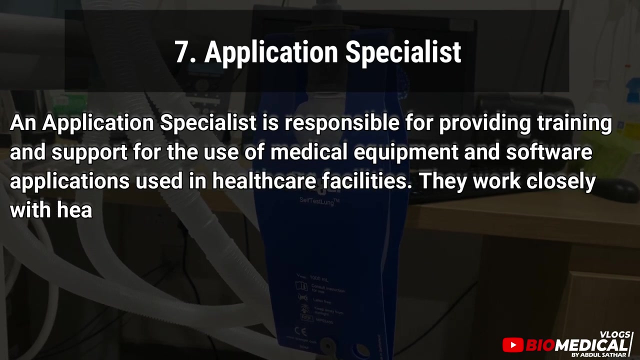 meet revenue targets and goals, etc. seven: application specialist. an application specialist is an application specialist who works in the field of health care, is responsible for providing training and support for the use of medical equipment and software applications used in health care facilities. they work closely with health care professionals to ensure that medical equipment and 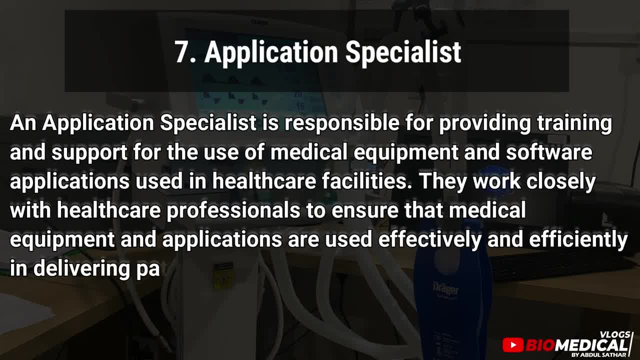 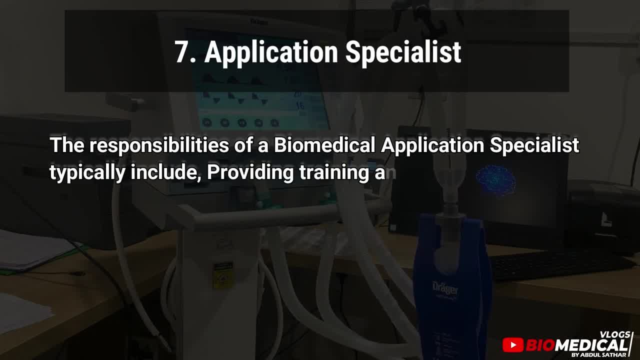 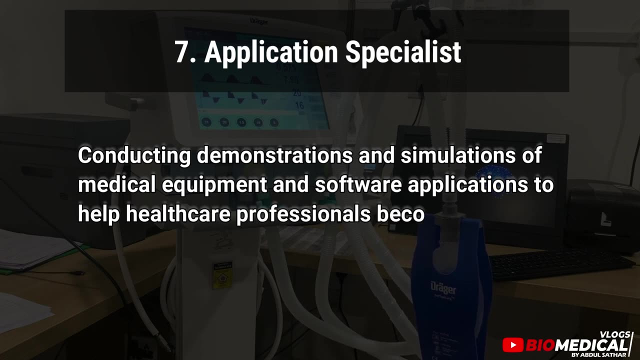 applications are used effectively and efficiently in delivering patient care. the responsibilities of a biomedical application specialist typically include: providing training and education to health care staff on the proper use of medical equipment and software applications. conducting demonstrations and simulations of medical equipment and software applications to help health care professionals become proficient in 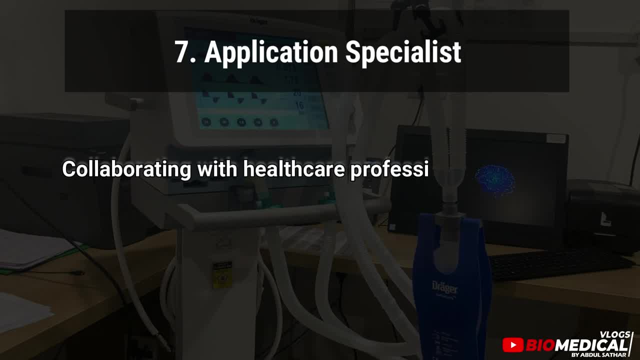 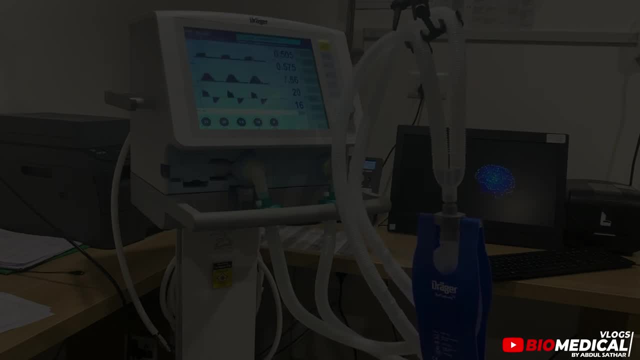 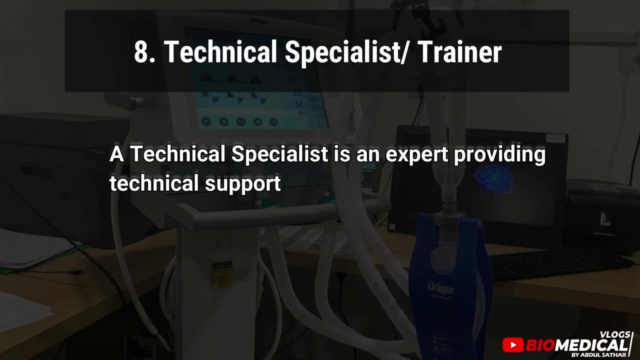 their use, collaborating with health care professionals such as physicians and nurses to identify training needs and provide customized training solutions. eight: technical specialist or trainer: a technical specialist is an expert providing technical support to the field service team, as well as providing escalation support and product service training to the engineers. 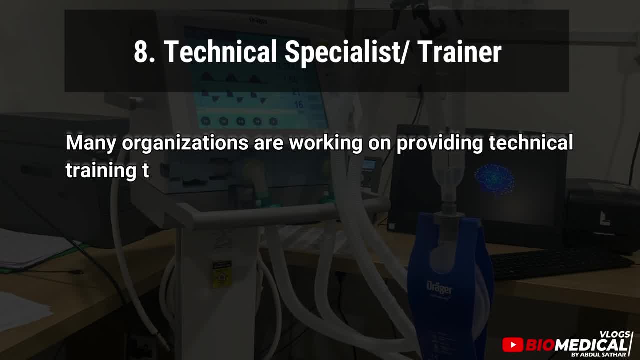 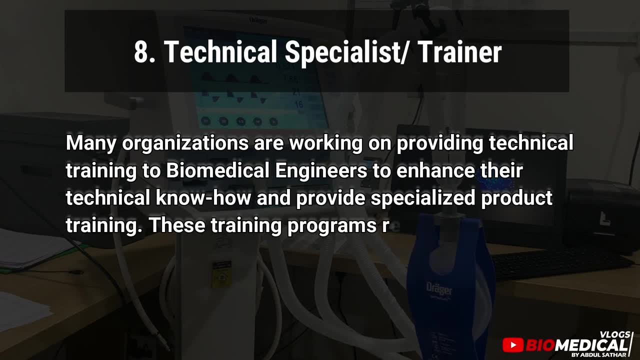 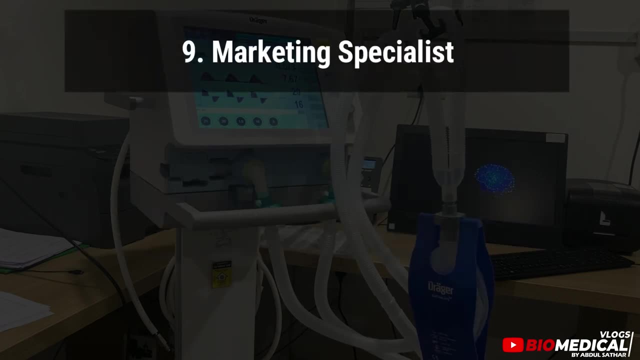 Many organizations are working on providing technical training to biomedical engineers to enhance their technical know-how and provide specialized product training. These training programs require skilled trainers to deliver the content effectively and facilitate learning. 9. Marketing Specialist. A marketing specialist is responsible for promoting medical devices and equipment to 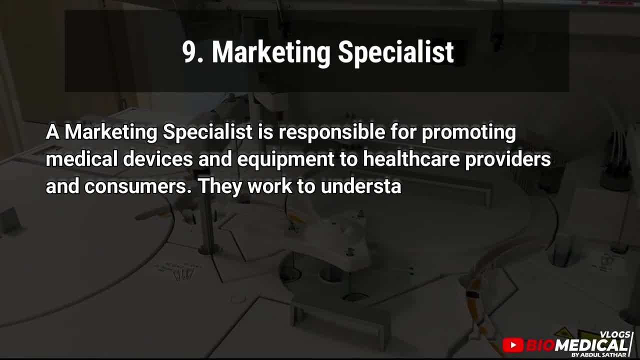 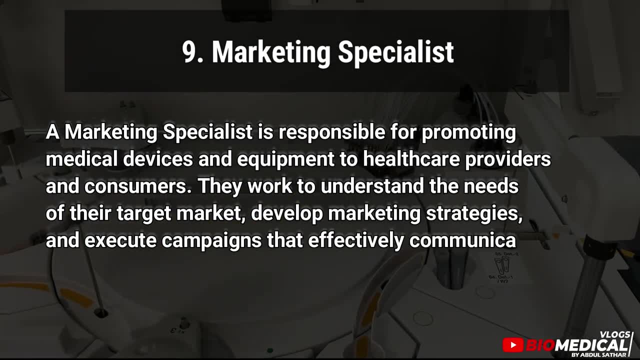 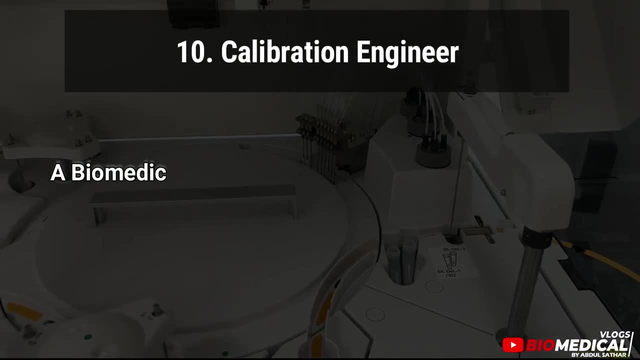 health care providers and consumers. They work to understand the needs of their target market, develop marketing strategies and execute campaigns that effectively communicate the benefits and features of medical devices. 10. Calibration Engineer. A biomedical calibration engineer is responsible for ensuring that medical devices and equipment. 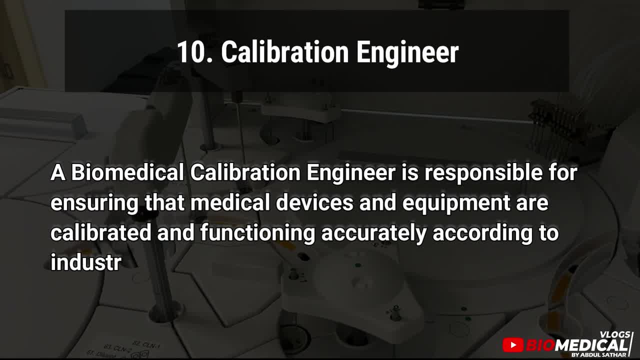 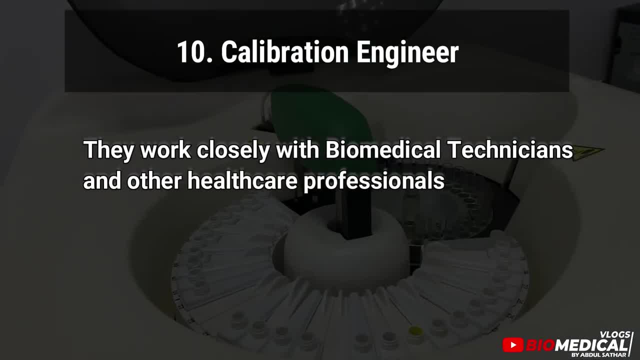 are calibrated and functioning accurately according to industry standards and regulations. They work closely with biomechanical engineers to ensure that medical devices are calibrated and functioning accurately according to industry standards and regulations. They work closely with biomedical technicians and other healthcare professionals to ensure that medical equipment is accurate, reliable and safe for use in patient care. 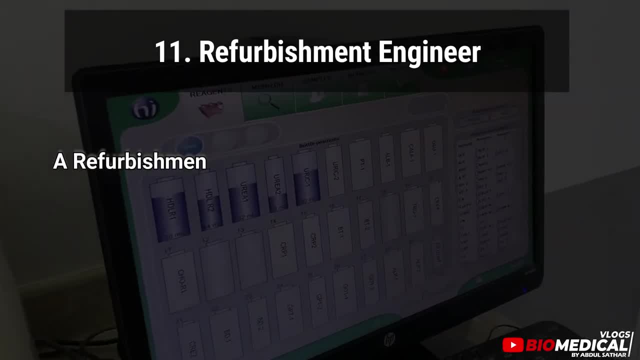 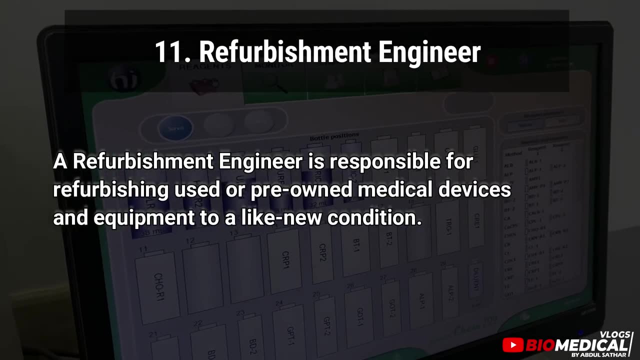 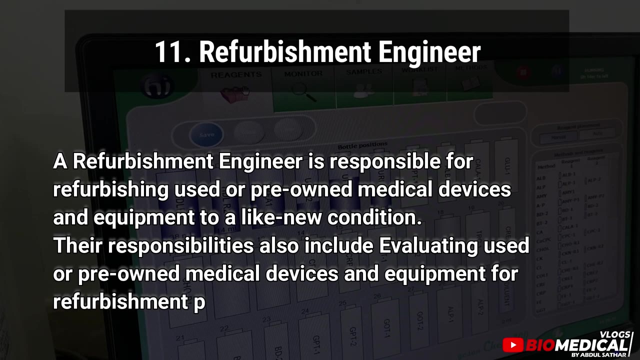 11. Refurbishment Engineer. A refurbishment engineer is responsible for refurbishing used or pre-owned medical devices and equipment to a like-nue condition. Their responsibilities also include evaluating used or pre-owned medical devices and equipment for refurbishment potential. 3. 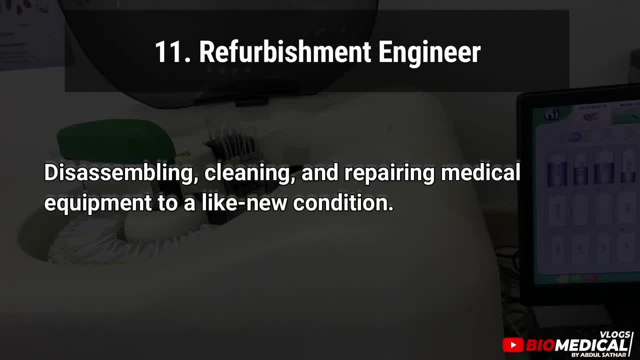 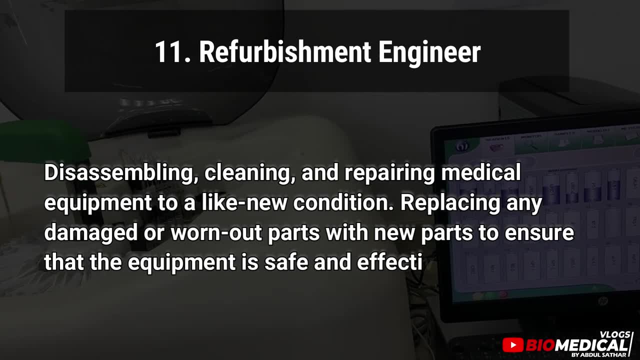 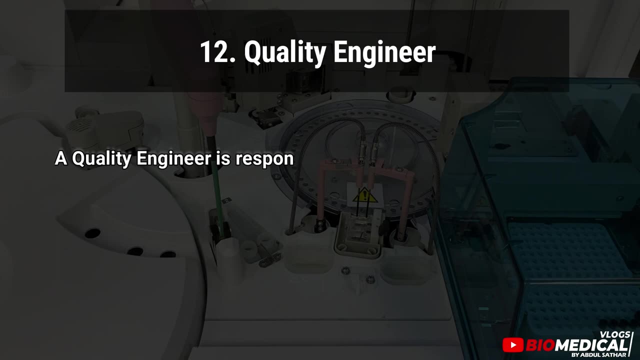 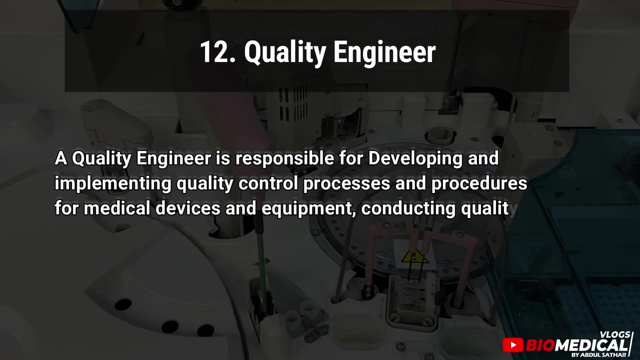 cleaning and repairing medical equipment to a like new condition, replacing any damaged or worn out parts with new parts to ensure that the equipment is safe and effective for use, etc. 12- quality engineer. a quality engineer is responsible for developing and implementing quality control processes and procedures for medical devices and equipment. conducting quality. 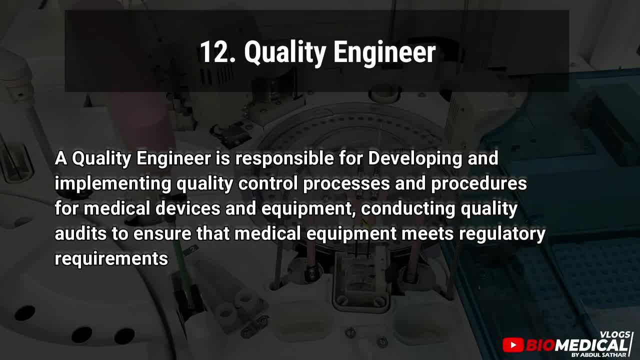 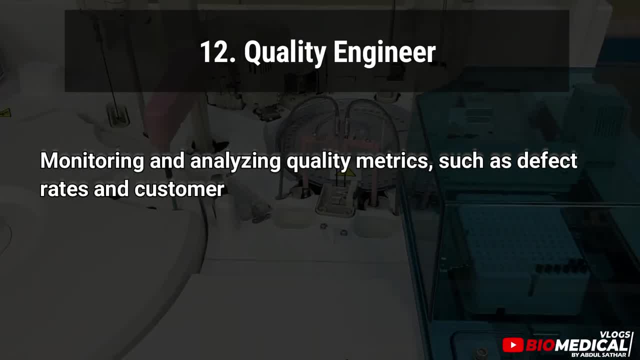 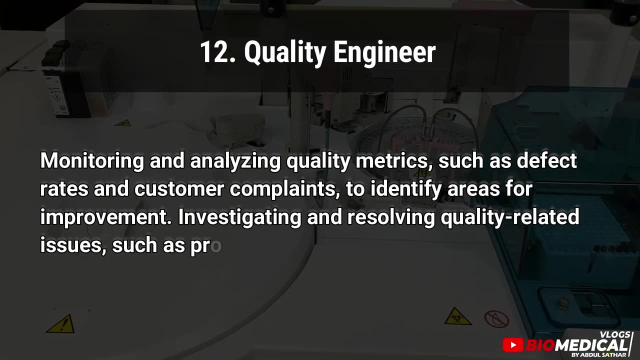 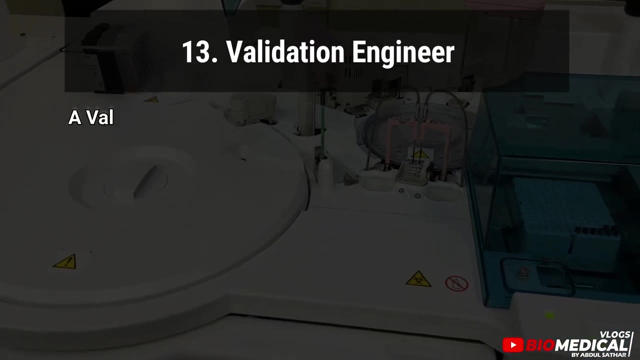 audits to ensure that medical equipment meets regulatory requirements and industry standards. monitoring and analyzing quality metrics, such as defect rates and customer complaints, to identify areas for improvement. investigating and resolving quality related issues, such as product defects and customer complaints. 13- validation engineer. a validation engineer is responsible developing and implementing validation processes and procedures. 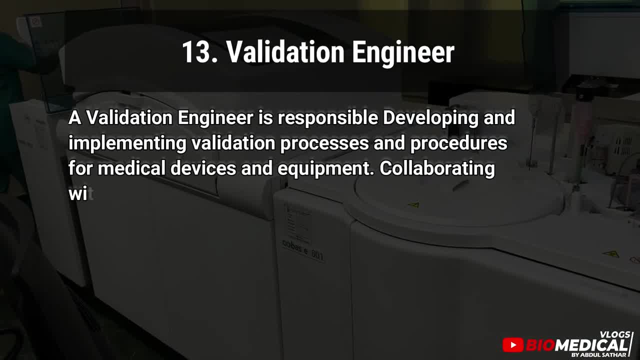 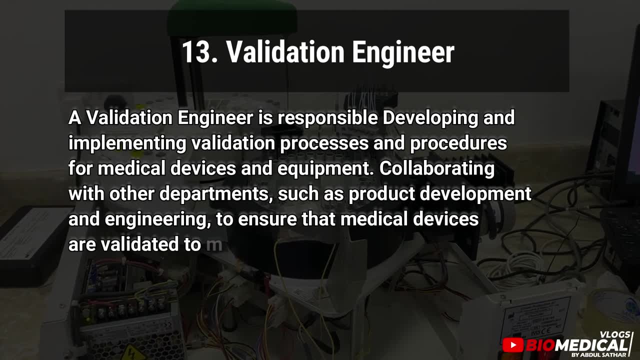 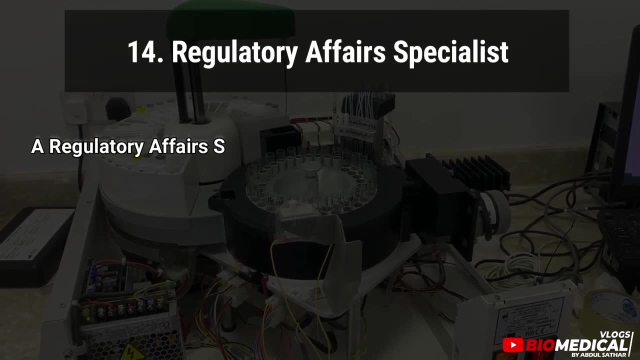 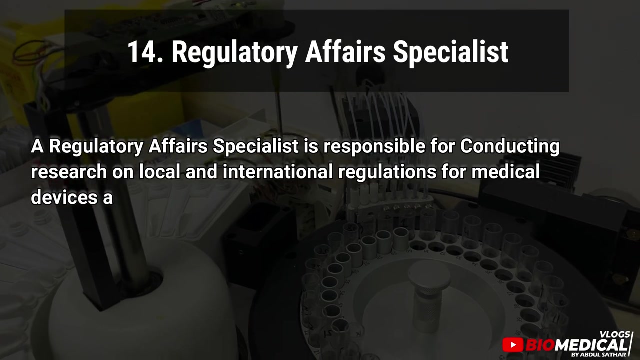 for medical devices and equipment, collaborating with other departments, such as product development and engineering, to ensure that medical devices are validated to meet quality standards. 14: regulatory affairs specialist. a regulatory affairs specialist is responsible for conducting research on local and international regulations for medical devices and equipment, preparing and submitting regulatory 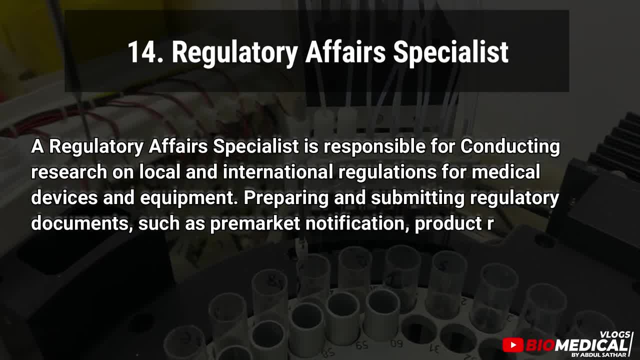 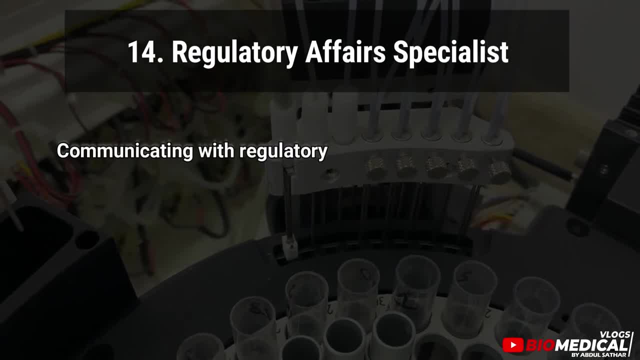 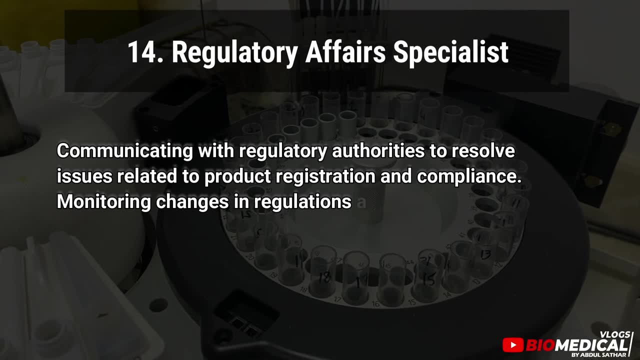 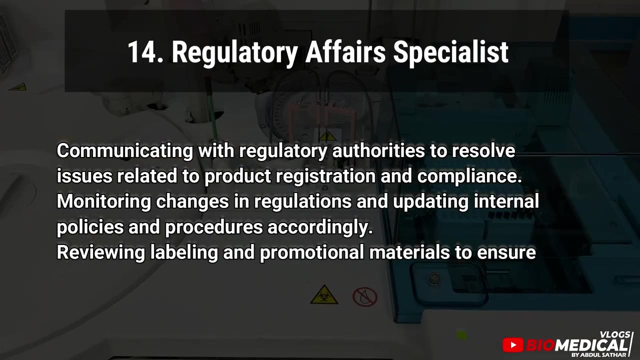 documents such as pre-market notifications and certification, product registration and technical files to regulatory authorities. communicating with regulatory authorities to resolve issues related to product registration and compliance. monitoring changes in regulations and updating internal policies and procedures accordingly. reviewing labeling and promotional materials to ensure compliance with regulatory requirements. 15- manufacturing engineer. 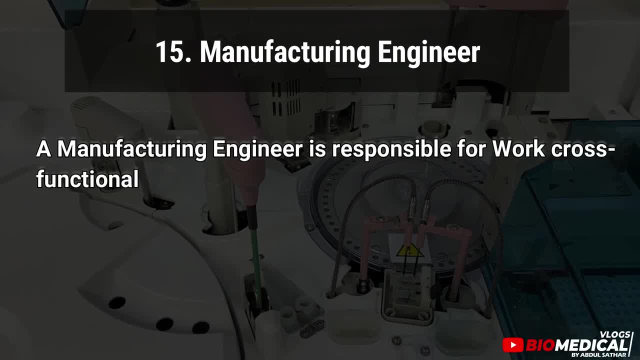 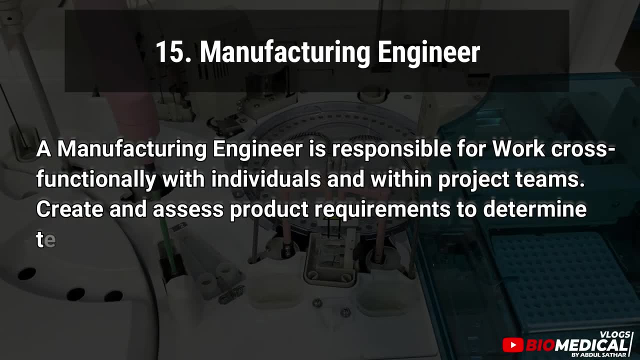 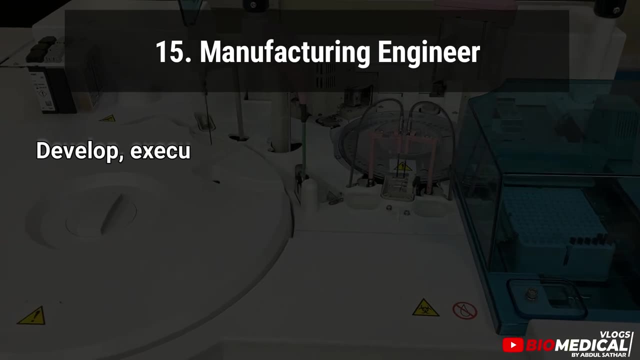 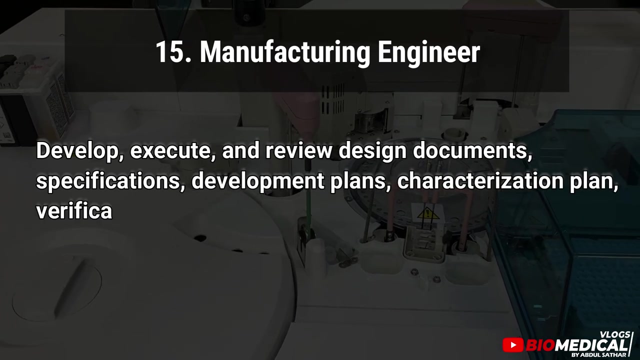 a manufacturing engineer is responsible for work cross-functionally with individuals and within project teams. create and assess product requirements to determine technical coverage and proper integration. perform design analyses and assessments. develop, execute and review design documents, specifications, development plans, characterization plan, verification plans, reports and other related product development documents for assigned 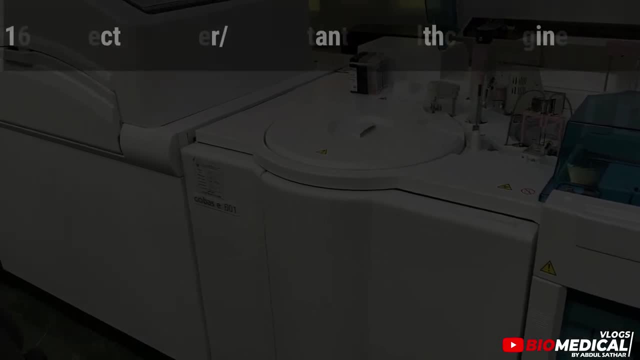 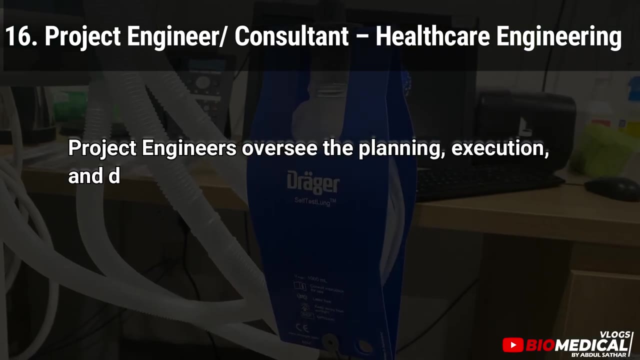 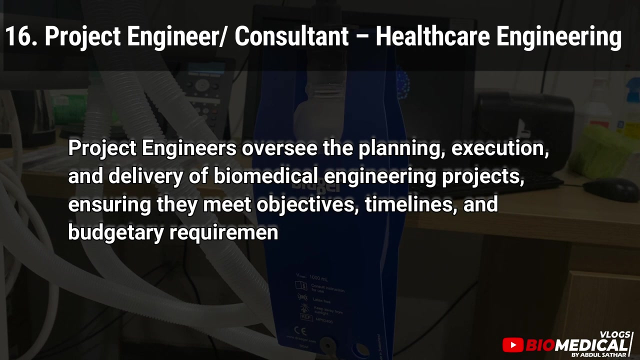 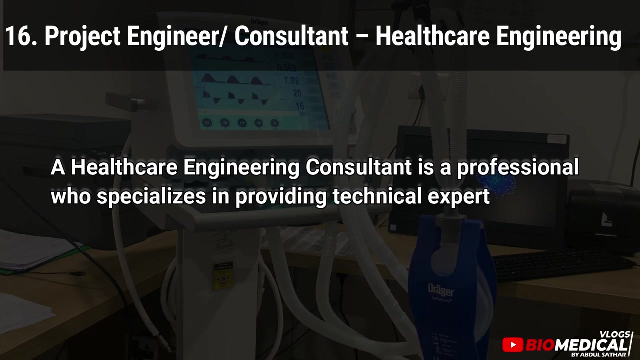 projects 16. project engineer or consultant. healthcare engineering project engineers oversee the planning, execution and delivery of biomedical engineering projects, ensuring they meet objectives, timelines and budgetary requirements. a healthcare engineering consultant is a professional who specializes in providing technical expertise and guidance to healthcare organizations. they use engineering techniques such as process mapping. 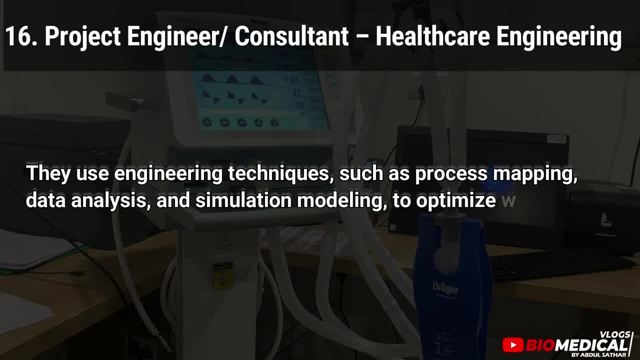 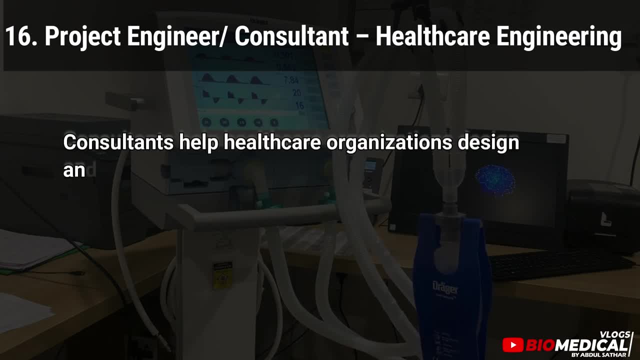 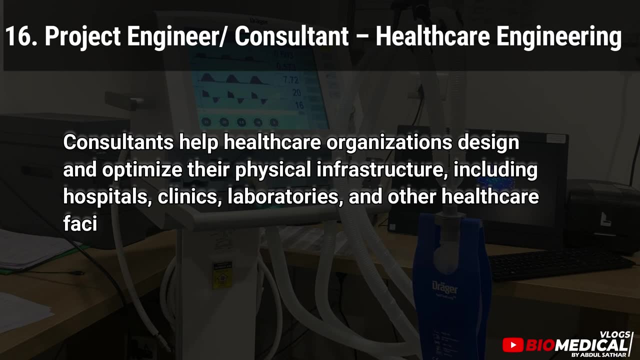 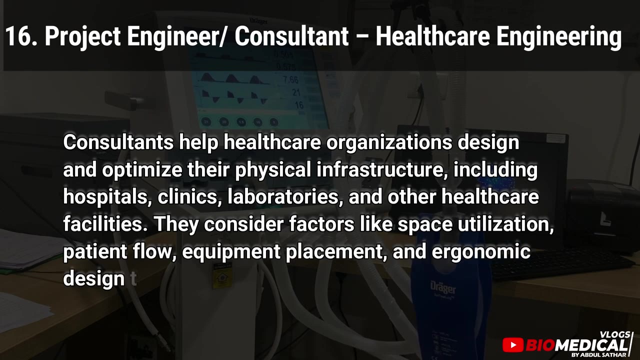 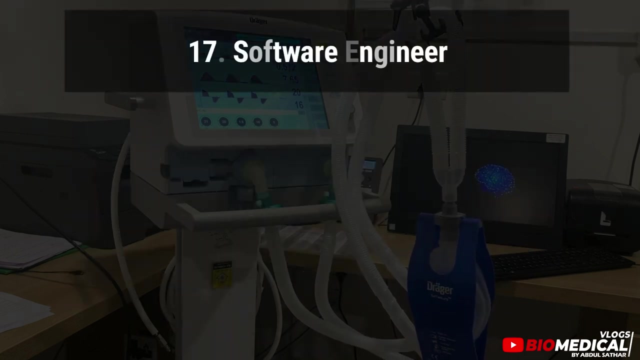 data analysis and simulation modeling to optimize workflows and enhance operational efficiency. consultants help healthcare organizations design and optimize their physical infrastructure, including hospitals, clinics, laboratories and other healthcare facilities. they consider factors like space utilization, patient flow, equipment placement and ergonomic design to create efficient and effective healthcare environments. 17. software engineer. a software engineer is responsible for 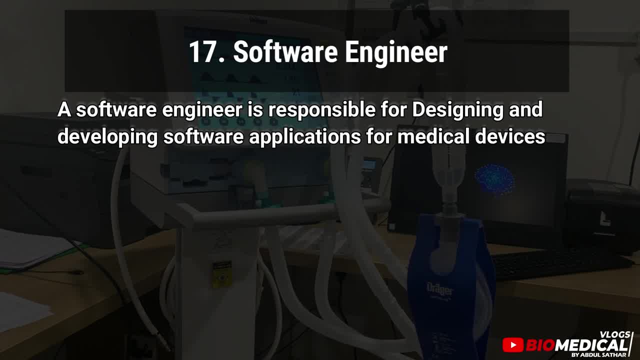 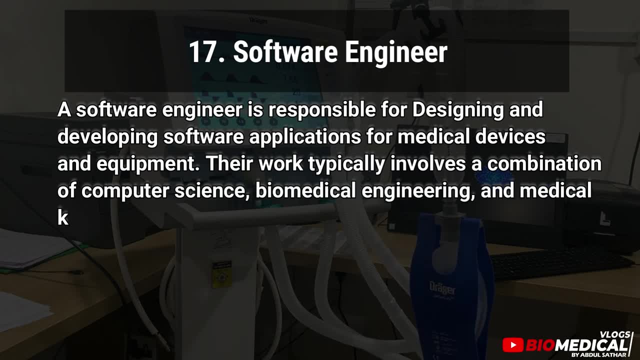 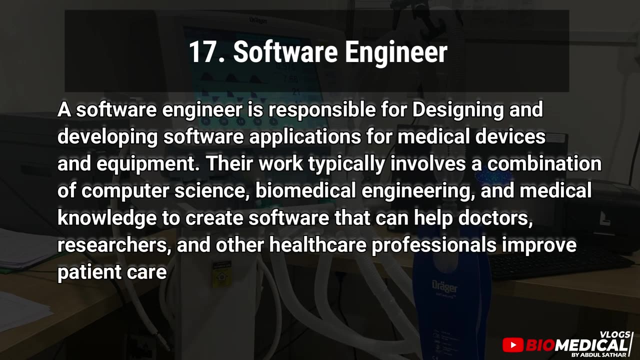 designing and developing software applications for medical devices and equipment. their work typically involves a combination of computer science, biomedical engineering and medical knowledge to create software that can help doctors, researchers and other healthcare professionals improve patient care and outcomes. conducting research on new systems can be a key area of development for healthcare professionals that are committed to 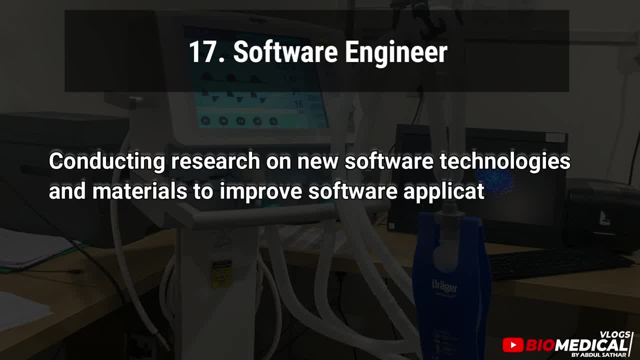 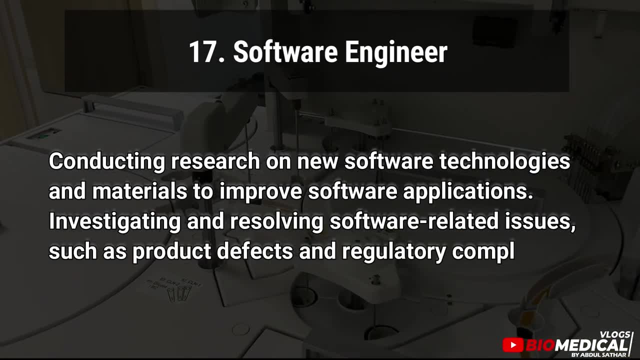 promoting and operating drinks and medical. Either software engineering or software engineering can produce an effective healthcare environment. software technologies and materials to improve software applications. Investigating and resolving software-related issues, such as product defects and regulatory compliance. Eighteenth Telephonic Support Engineer. 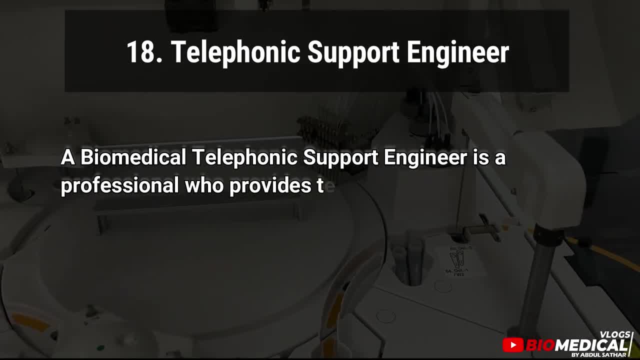 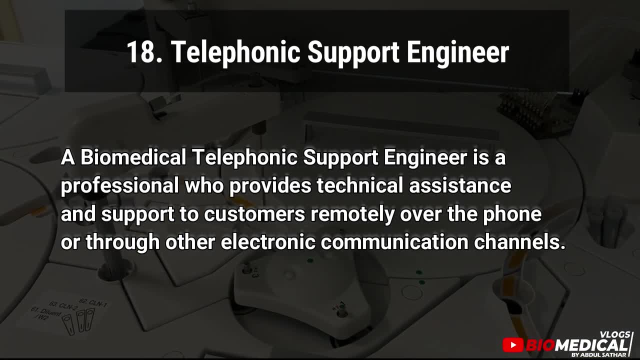 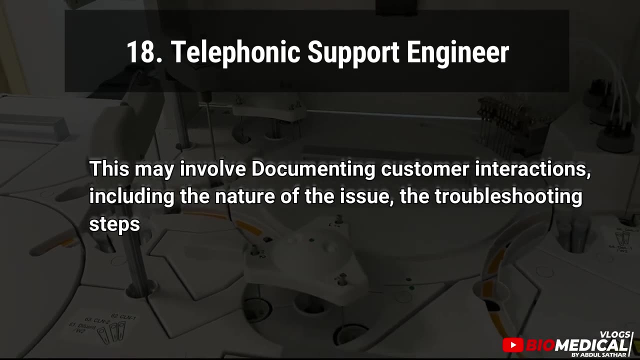 A biomedical telephonic support engineer is a professional who provides technical assistance and support to customers remotely over the phone or through other electronic communication channels. This may involve documenting customer interactions, including the nature of the issue, the troubleshooting steps taken and the resolution of the problem. 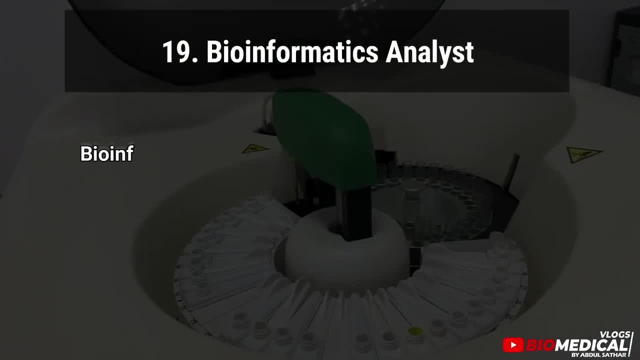 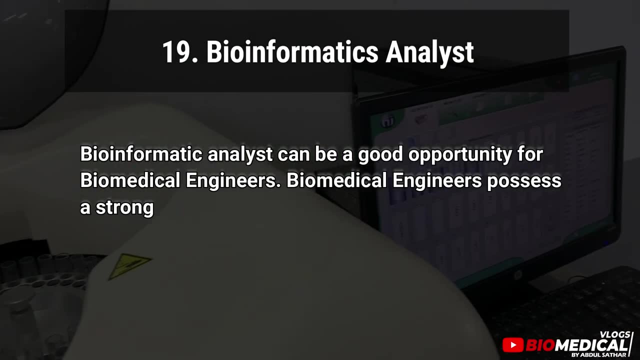 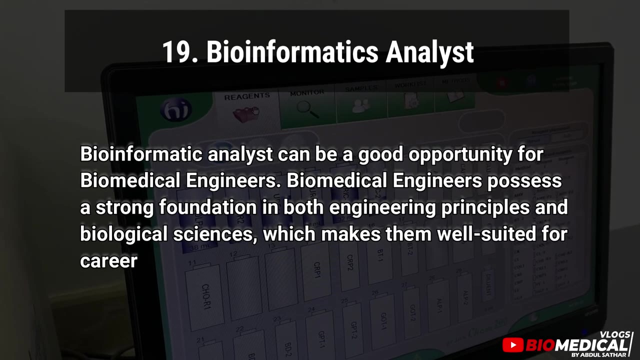 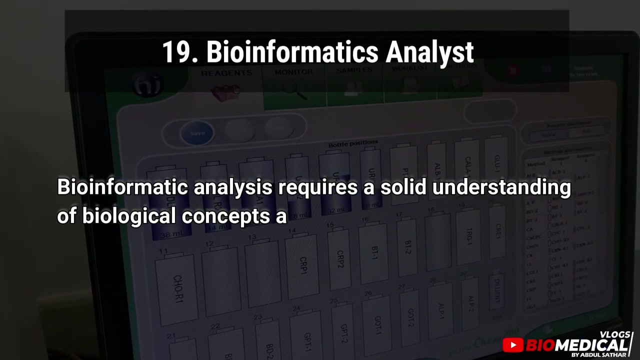 Nineteenth Bioinformatics Analyst. Bioinformatics Analyst can be a good opportunity for biomedical engineers. Biomedical engineers possess a strong foundation in both engineering principles and biological sciences, which makes them well-suited for careers in bioinformatics. Bioinformatic analysis requires a solid understanding of biological concepts and experimental techniques. 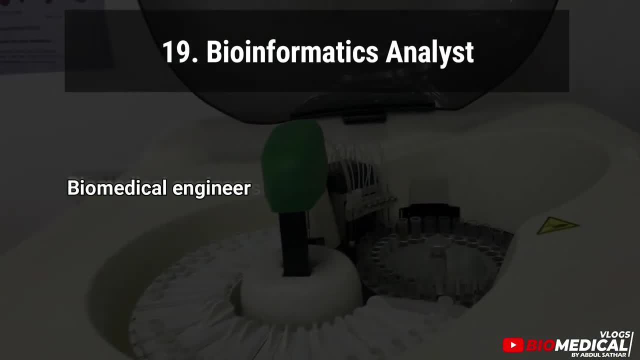 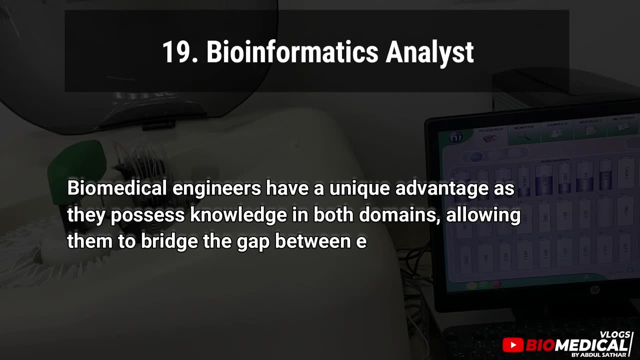 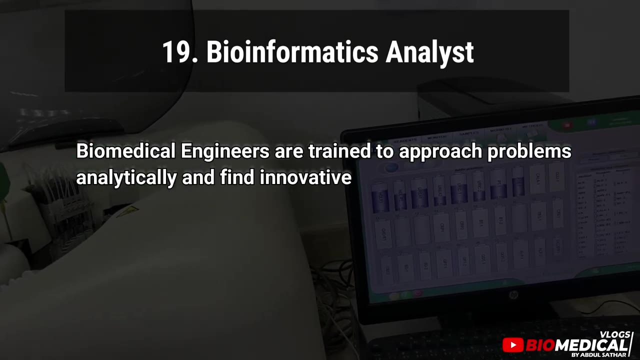 combined with computational skills. Biomedical engineers have a unique advantage as they possess knowledge in both domains, allowing them to bridge the gap between engineering and biology. Biomedical engineers are trained to approach problems analytically and find innovative solutions. These skills are highly valuable in bioinformatics. 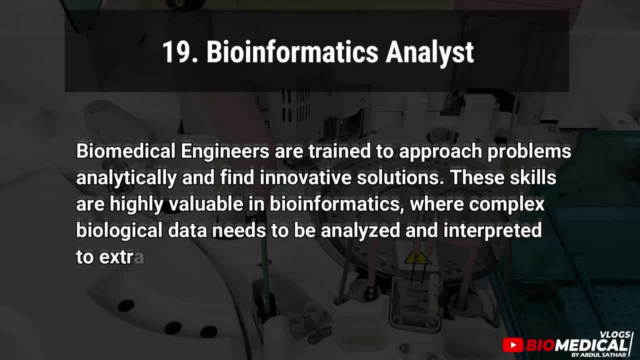 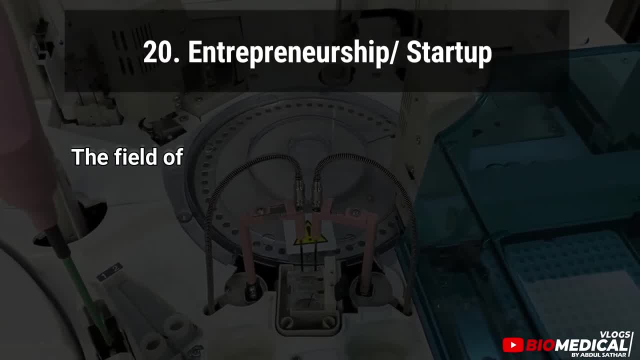 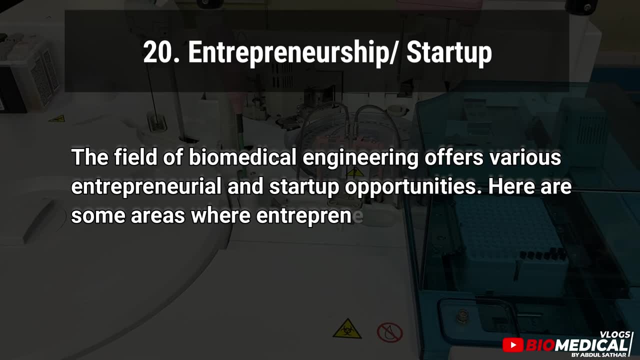 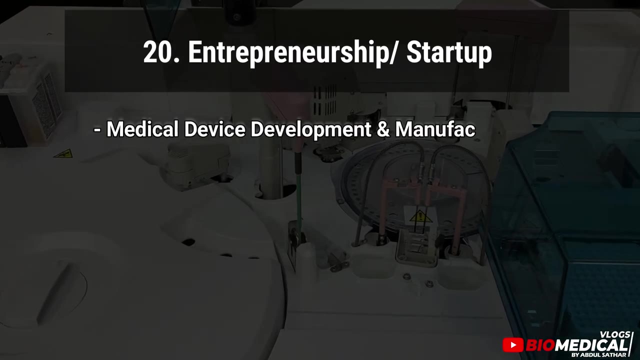 where complex biological data needs to be analyzed and interpreted to extract meaningful insights. Twenty: Entrepreneurship or Startup: The field of biomedical engineering offers various entrepreneurial and startup opportunities. Here are some areas where entrepreneurs can explore opportunities in biomedical engineering: Medical device development and manufacturing. 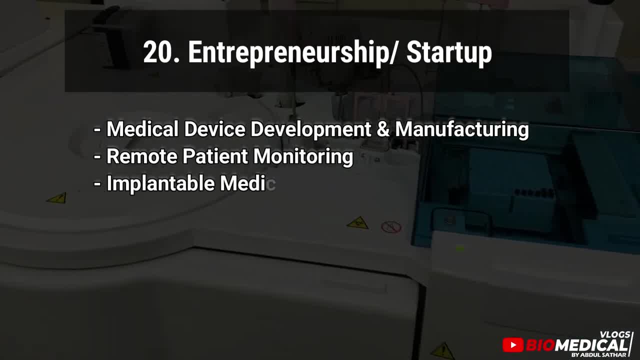 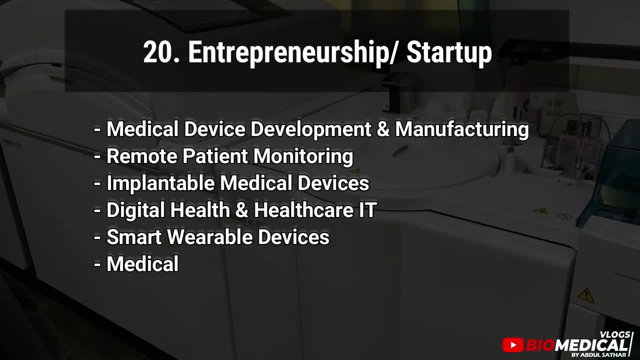 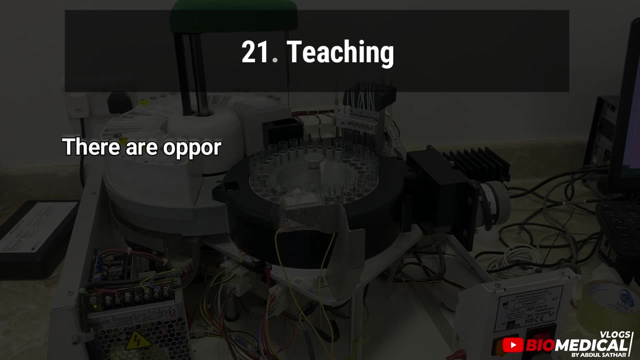 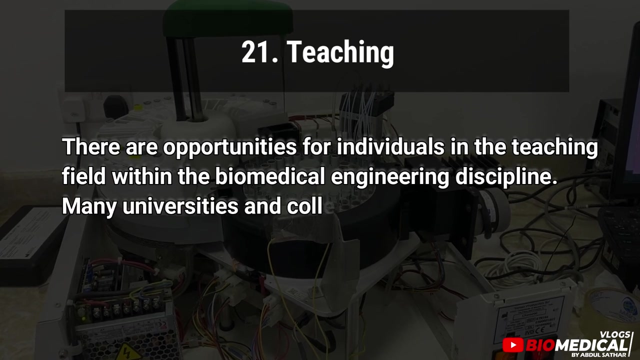 Remote patient monitoring, Implantable medical devices, Digital health and healthcare IT, Smart wearable devices, Medical device distribution, etc. Twenty-one Teaching: There are opportunities for individuals in the teaching field within the biomedical engineering discipline. Many universities and colleges offer biomedical engineering programs, where educators are needed to teach undergraduate and graduate courses.